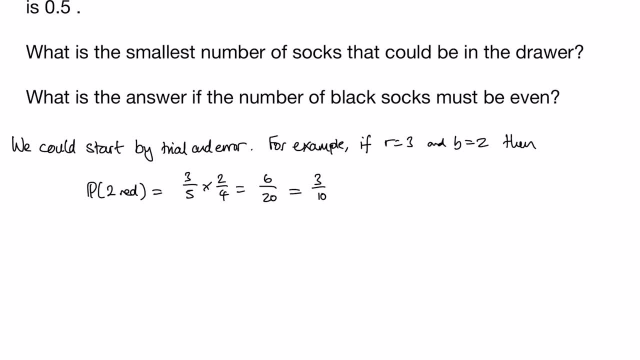 total. So that's 6 20ths or 3 tenths. It doesn't take too long to find that if the number of black socks is 1 and the number of red socks is 3, that we have the probability of two red is 3 quarters. 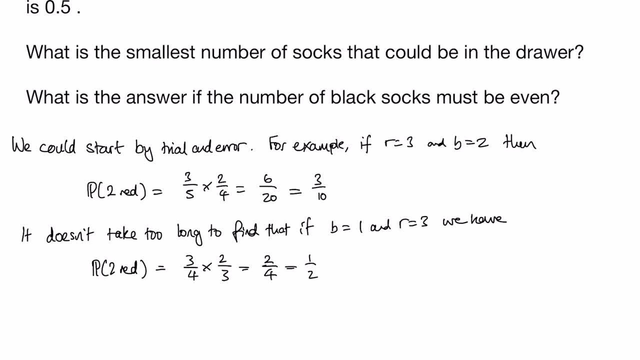 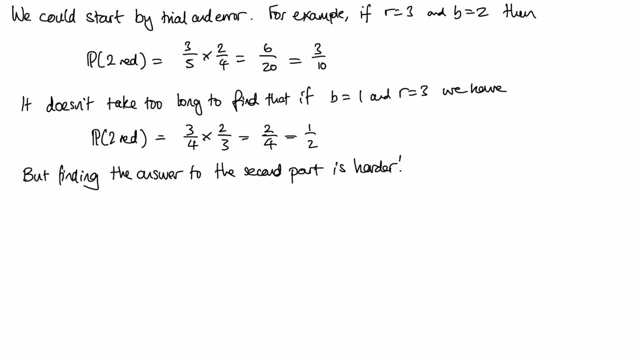 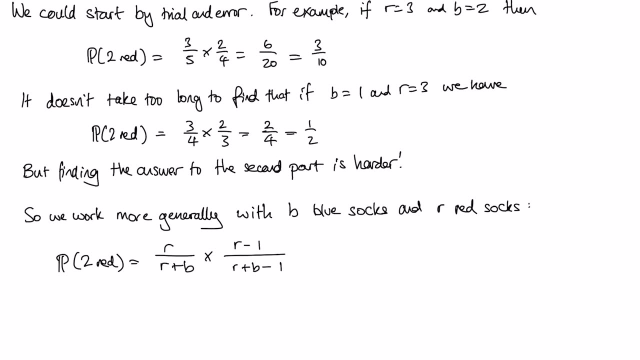 2 fourths or 1 half. So we get the answer quite quickly by trial and error. but finding the answer to the second part is a lot harder. So we work more generally with b- blue socks and r- red socks and we find the probability that we have two red socks would be r divided by r plus b Initially. 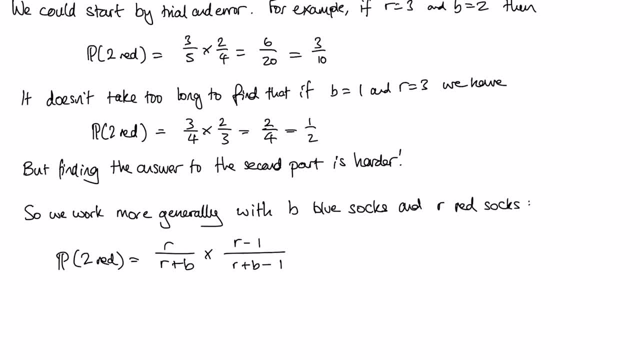 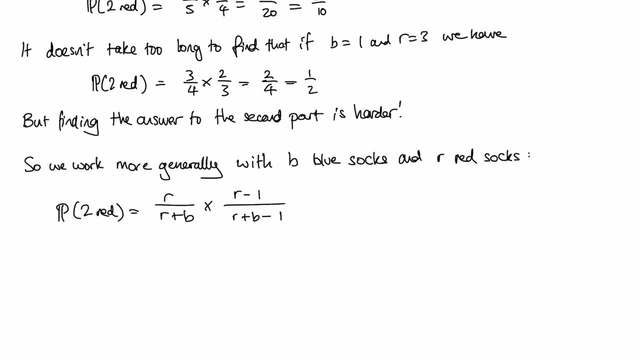 there are r red socks and r plus b socks in total and then once we've taken one red sock, we would have r minus 1 red socks and r plus b minus 1 socks in total. so we get that second fraction there and we multiply to find the probability that both socks 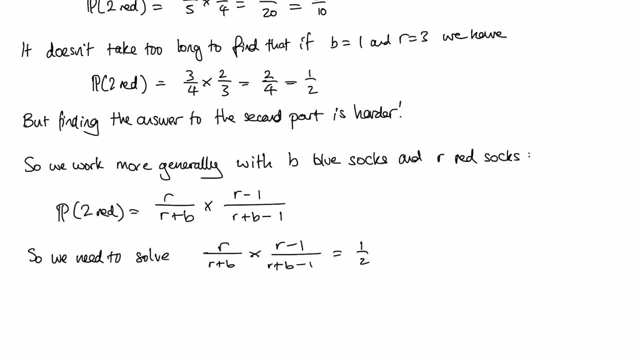 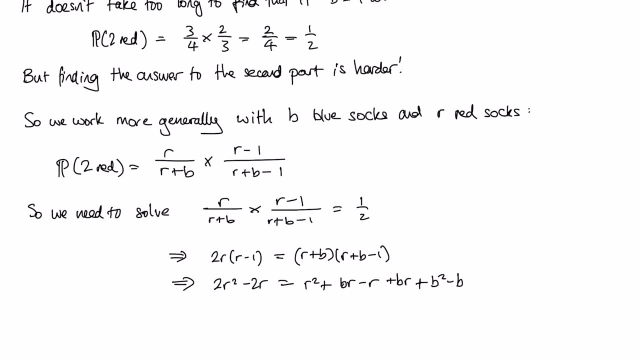 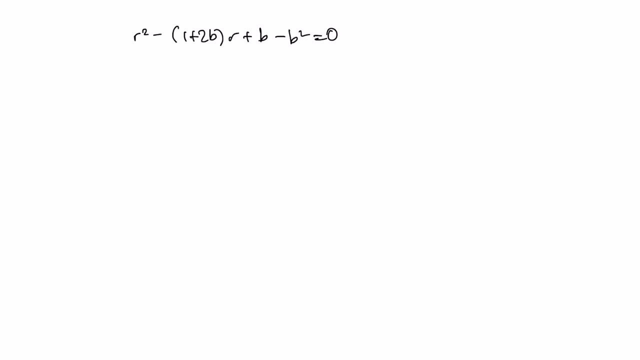 are red. So we need to solve that expression as equal to a half. so we just do a little bit of algebra, some multiplying out and then refactorizing, so that we get the equation in the form of a quadratic equation in r. So once we've got that quadratic equation in r, we can just plug. 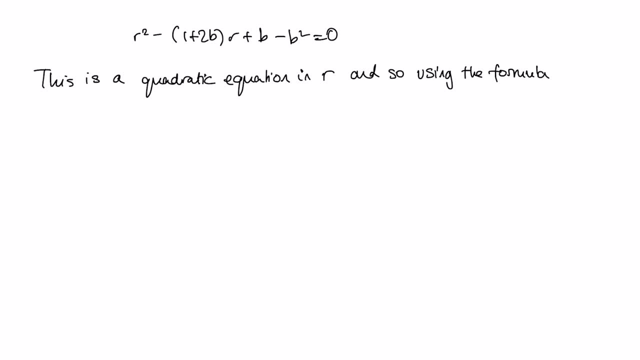 the coefficients into the quadratic formula, the coefficients being 1 minus 1 plus 2b and b plus b, squared in the usual places of a, b and c in the quadratic formula. So we do all of that multiplying out and simplifying, and we get this form: 1 plus 2b, plus or minus the square root of. 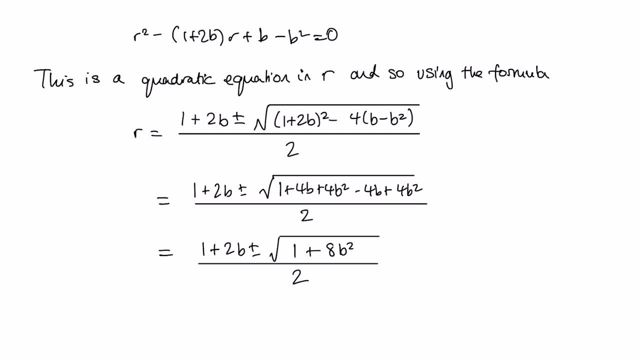 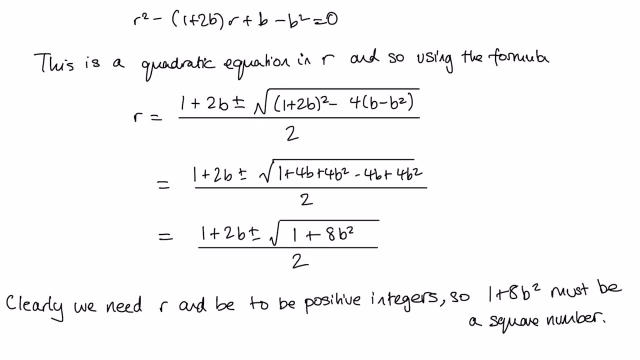 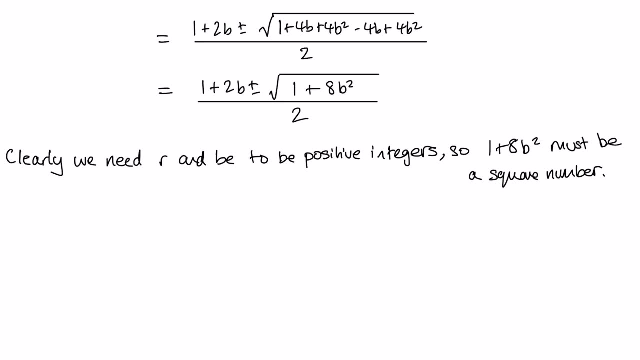 1 plus 8b squared over 2.. In fact we'll only be interested in the plus solutions that give us positive numbers here. So clearly we need r and b to be positive integers. so it must be that 1 plus 8b squared must be a square number, so that when I take that square root I get a whole number. 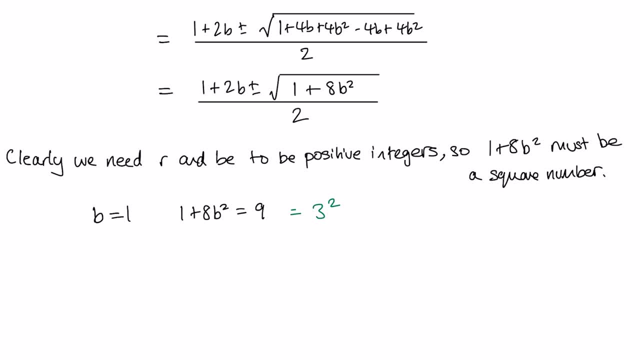 So if we take b equals 1 plus 8b squared, we get a square number, so that when I take that square root of 1, we get 1 plus 8b. squared is 9, that's 3 squared, and that gives us the solution that we. 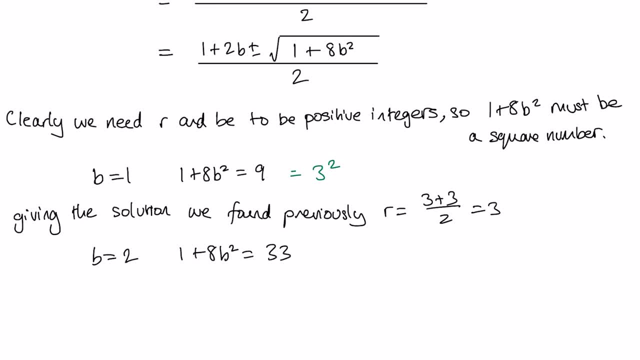 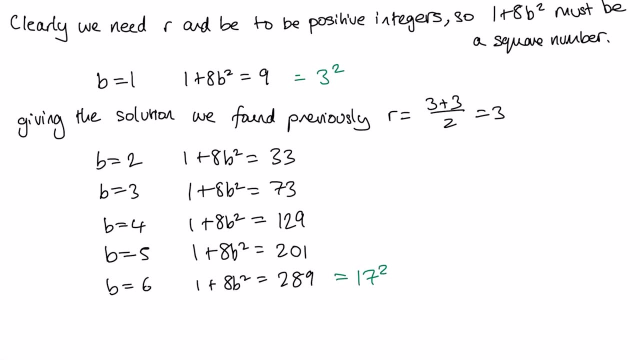 found previously, and we can try a few more values for b, 2,, 3,, 4,, 5, until we get to 6,, which is the next time we get a square number- 17 squared- and so that gives us the solution. 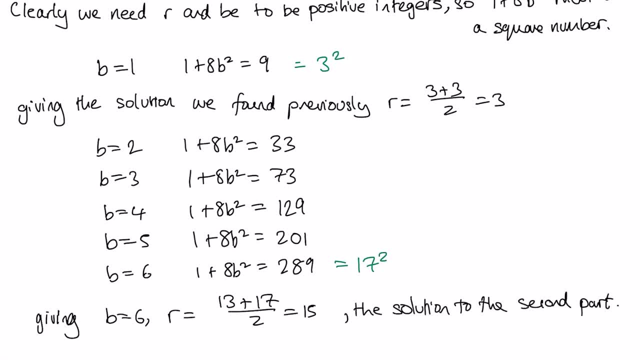 to the second part: b equals 6, and r is equal to 13 plus 17 over 2,, putting it back into the formula, which is 15,, and so that's the solution to the second part.